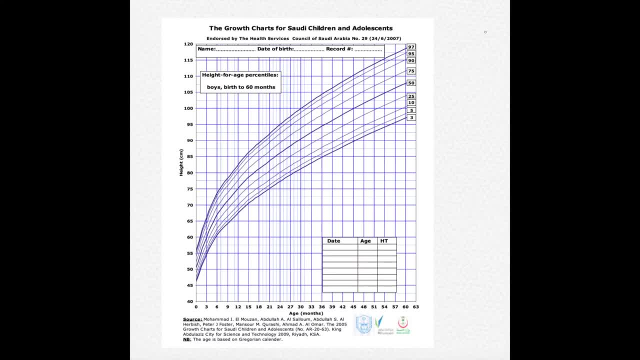 thing you should check first in any growth chart. so if you have a child, one year old child has height as in centimeters, as 70 centimeter. how are you gonna displace that on the chart? okay, so his age is one year, as you can see here in month 12. okay, and you can go up up here till you meet up with. 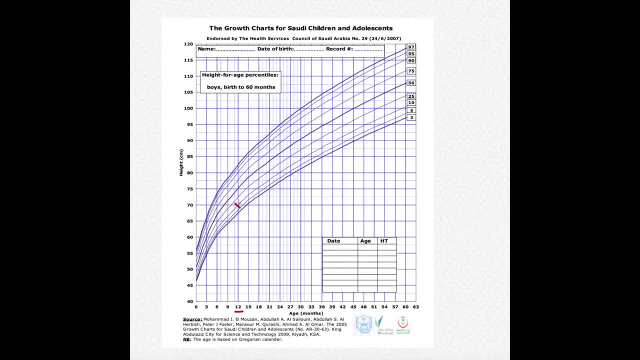 a 70. okay, you should droll, I can X or like, you also can drool, like adapt, okay. so after this, this is the first thing you can check, and that's where my child is 107 years old. Chavez could see me as 70. Tôi ko tHay là cái 100께서kop k. 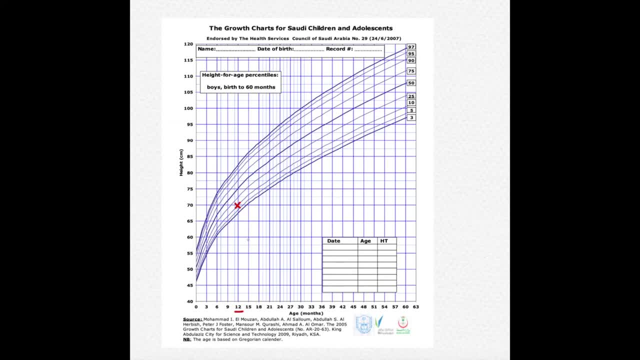 alright, so this I had three. you can see the capitalism of the system, like the system do. okay, let's say, we have another child in the blue, one, uh, let me, yeah, in the blue. okay, one years old too, but the baby in the blue, he's like here. and we have another child, the green child. 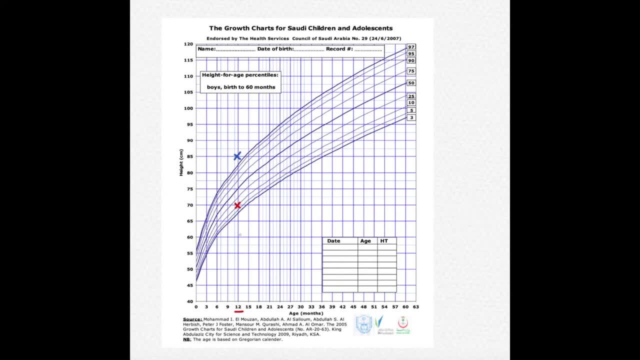 his uh, his uh. his height is like 60 here. they're all the same age, they're all one year old, but they just play in the chart in the different, in the different site. okay, so how we can interpret this? so first you can see this. okay, let me draw it in red. you can see the line from here. 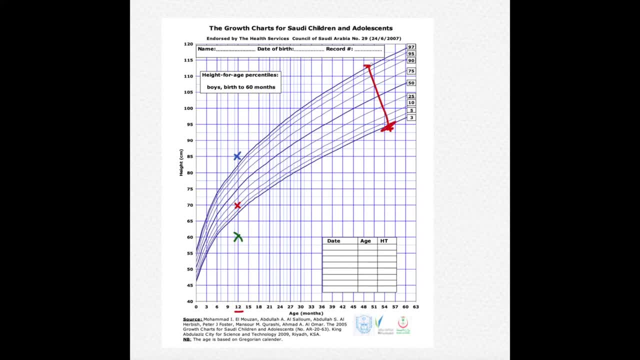 till here, right till here, right. so this is the normal. so whenever, whatever is its display here, or wherever x or dot you you put inside here, it will be normal okay. so, child in the red one, in the x, he's normal, okay. and the child is on the blue one: he's higher than normal, taller than normal. 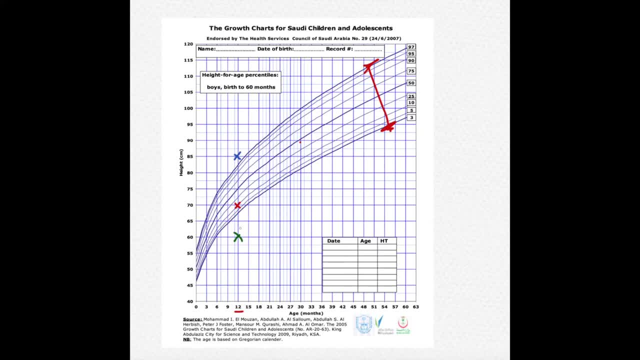 okay, higher, i mean taller than no. okay, and the child in in the green x, he's shorter than normal, so below that, the the this graph below this, like the graph from here to here: below it is short, above it is tall, okay, and also it's display as well as for head circumference if it's. 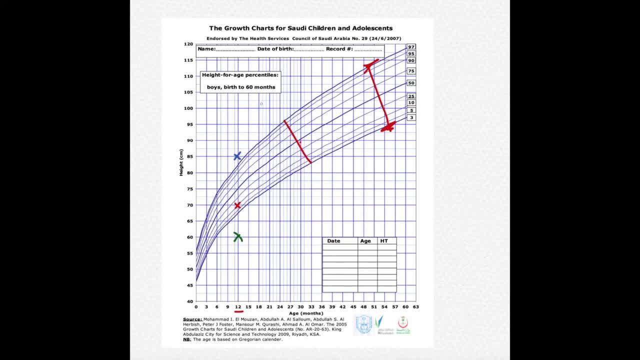 if it's above here, it's mean the baby had a big head and like macro, uh cephaly. or if the patient is uh under the curve, uh, like the green one here, you should know he has a micro syphilis. okay, so we have different, also for weight. if he's display here, that means he's normal. if it's above, it's. 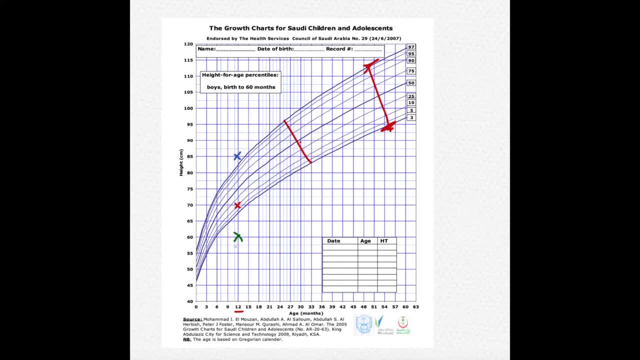 he's uh bigger than normal. if it's uh below the curve, he's smaller than normal. so after we finish this, uh, you should track that, the x like the red x, like we can see here, and when you track it down here, you will end up with 10. what does that mean? what does this number? 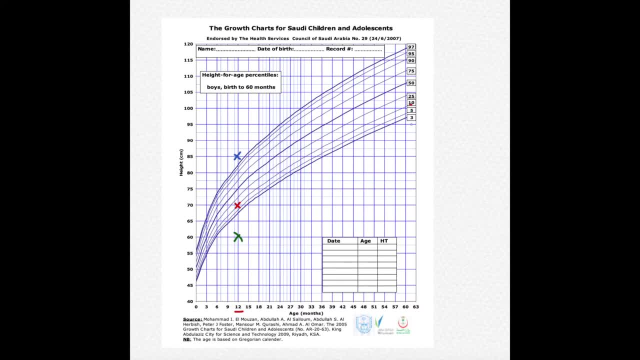 mean this number display: 100 kit. okay, 100 child. so your child is gonna be number 10.. nine of the children, nine of the children- will be shorter than him and 90 percent- 90- will be like taller than taller than him. okay, so this is the way, just you know. 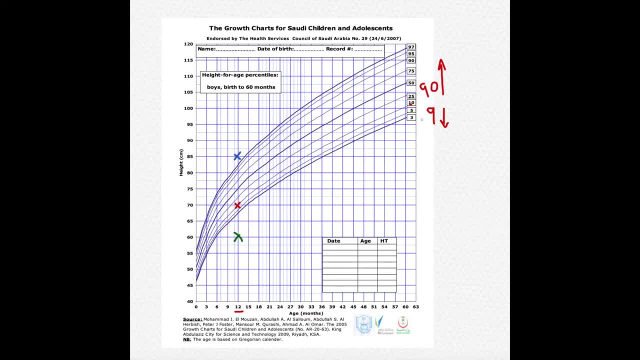 that the, the, the, not the percentage. that where your baby fall and to like according to his age and according to his uh like, uh uh other children in his age, like. as we see, if the patient is to play here, 50 that means 50 uh children will be uh like taller. 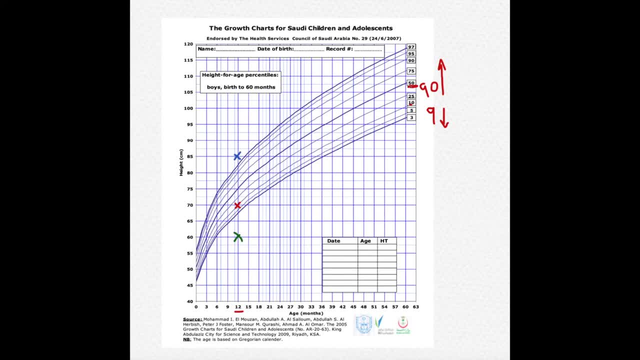 him and 50 will be, uh, shorter than him. so this is what the number here mean. so, as you can see, here we have, uh, the red and the green. here i just place it like: imagines two child. we have child and red and child and green. okay, uh, as you can see that the both. 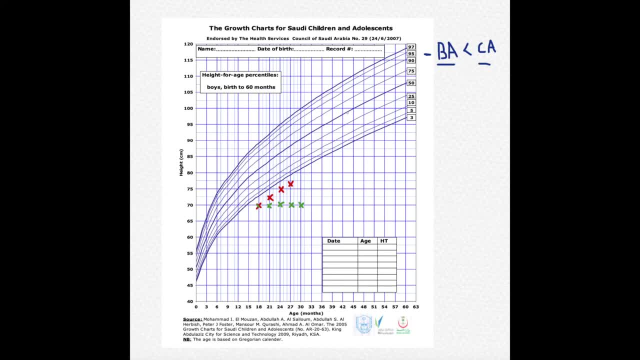 children are displayed below the the curve. that means here the children's are short. okay, so how we can interpret this. first, after you like you just place it on the chart. you should check the boon age of the child. okay, let's take an example. the boon age of the child is less than the 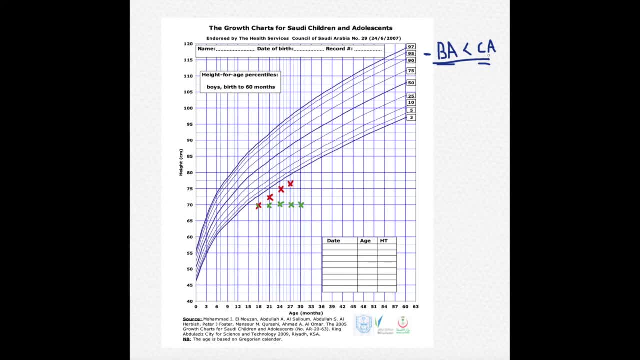 chronological age, that, what does that mean? the boon age? you check it in on x-ray. okay, so, uh, if you are a 10 years old child, your boon age, uh, normally it will be 10.. okay so, uh, if, if you find out that the, the, the, the red one, the red one is the boon age of the child, uh, then you can. 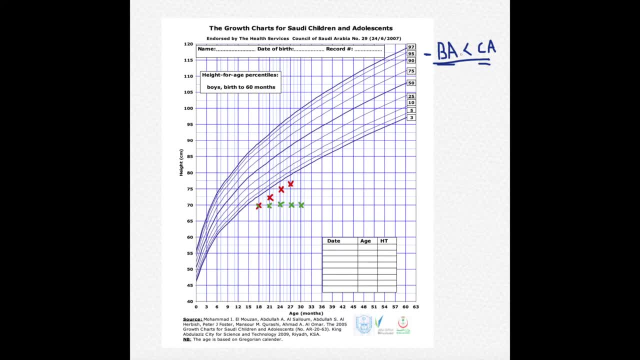 see that the red child and the green child, uh, have less the boon a. their boon age is less than the chronological age. that mean different thing. okay, after you see this, after you see this, you should check: is the baby going with the curve? the velocity is it going with the curve as you see in? 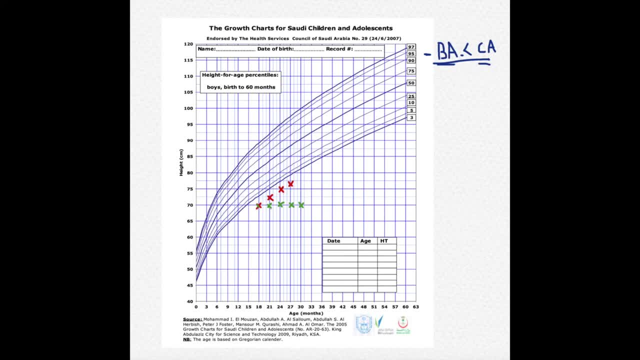 the red child here and if it's not going with the curve, as you see in the green one, if it's going with the curve, that mean different thing. that's mean maybe the baby must have problem with the boon age and that's probably is the constitutional delay that mean the child here. let me just do it. 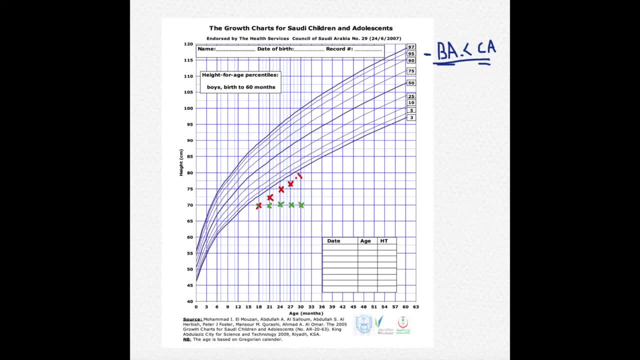 in red. the child here will eventually, will eventually jump to the normal. okay, he will jump, it's a normal delay, constitutional delay from its name, constitutional delay, okay. and what about the the the green one? okay, you should check the boon age and it's, it's lesser than the chronological. 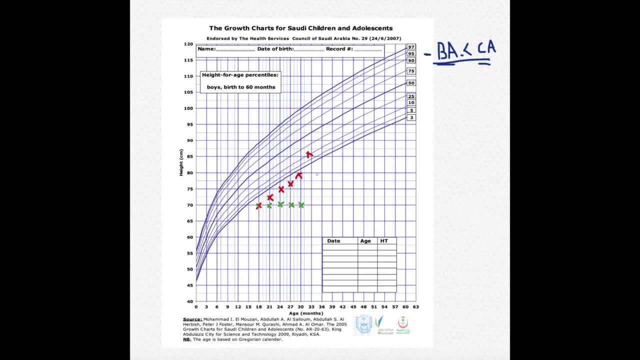 age. what does that mean? the green, the green one, it's not going with the curve, it's not the, it's like as you see here, it's not like the velocity here in red. what does that mean? that mean the baby have different things, maybe chronic illnesses like 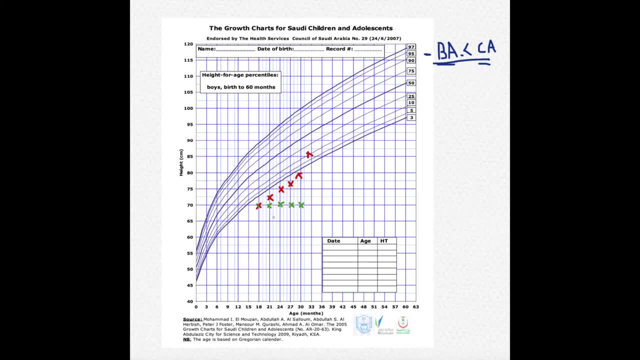 chronic renal failure. maybe he have nutritional problem, like gastrointestinal, like celiac or Crohn's, okay, and maybe endocrine abnormality, like a growth hormone deficiency or hypothyroidism. so what if the Boone age is equal to the chronological age? that mean also two things: is it going with the curve? the? 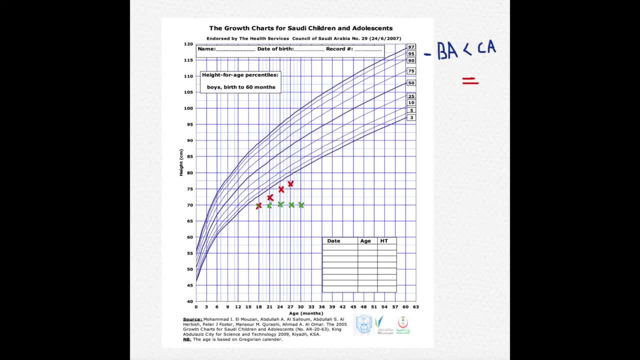 velocity, normal or not, like the green one, okay, if it's equal. if you see the child here, have that the, the Boone age is equal, the chronological age and he's going with the curve, that mean most probably familiar cause. you can see, like the child, his family predicted range is here. so the child will grow eventually here.